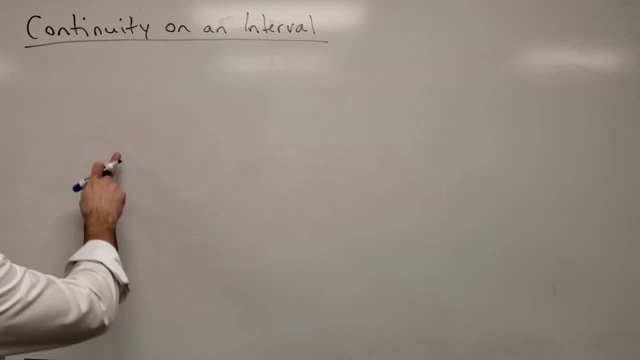 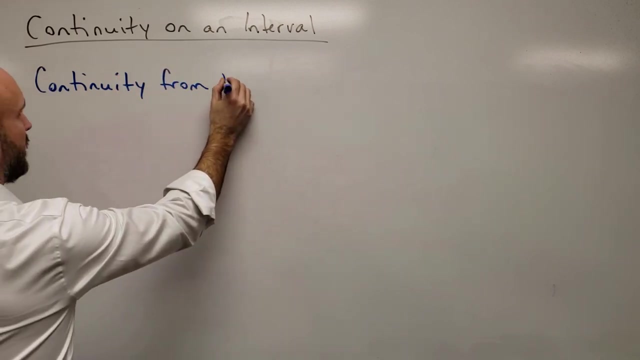 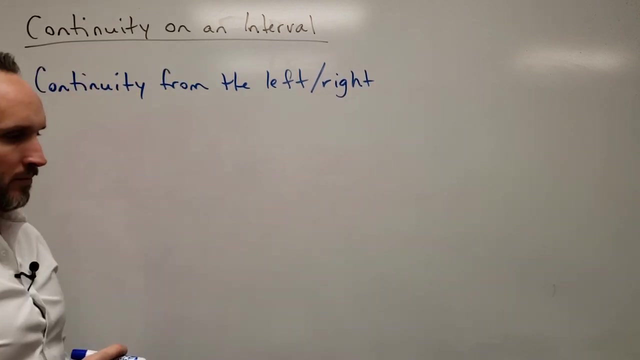 from the left and continuity from the right. So let's talk about continuity from the left or right first. So continuity at a value means continuity from both sides. So if we say f is continuous from continuity from both sides, then we have continuity from both sides. So if we say 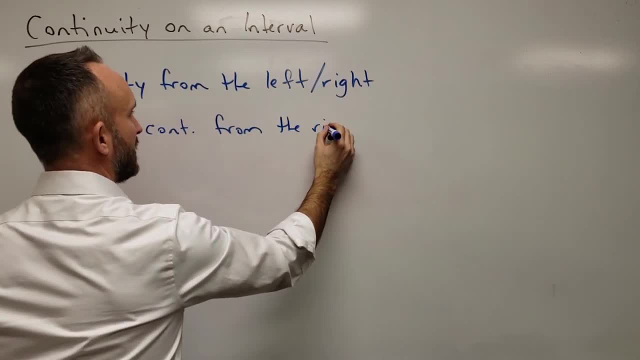 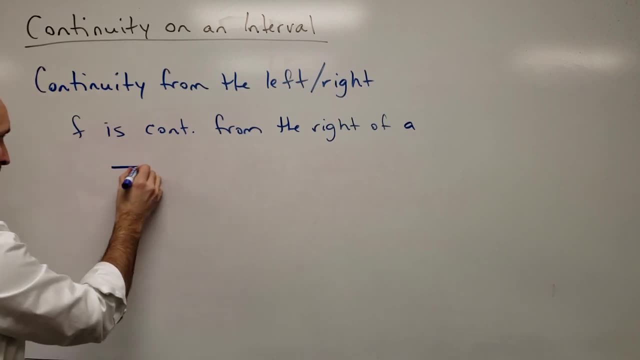 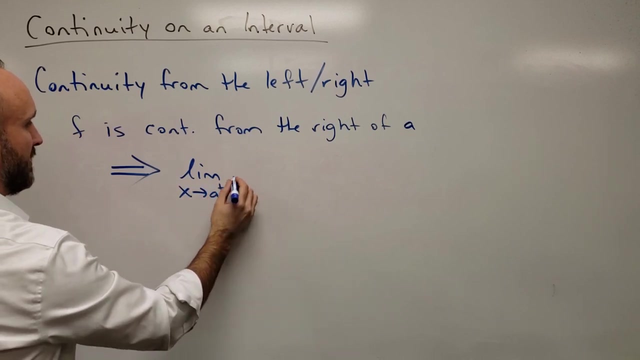 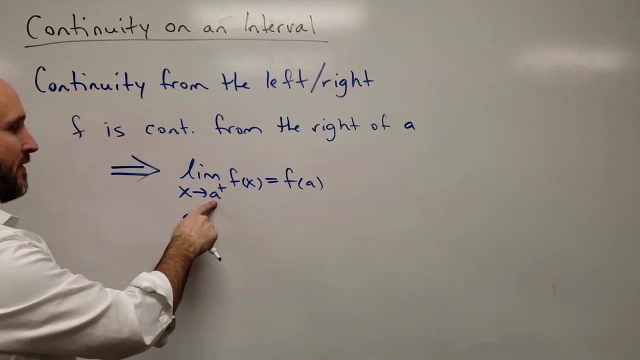 f is continuous from the right of a value, let's say f is continuous from the right of a. well, that means that the limit as x approaches a from the right of f of x equals the output of the function at a. So instead of just approaching a from both sides, 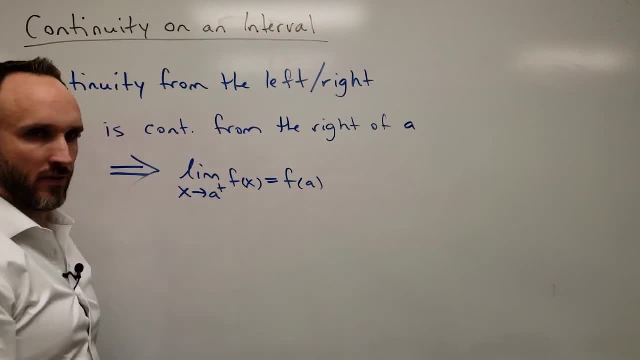 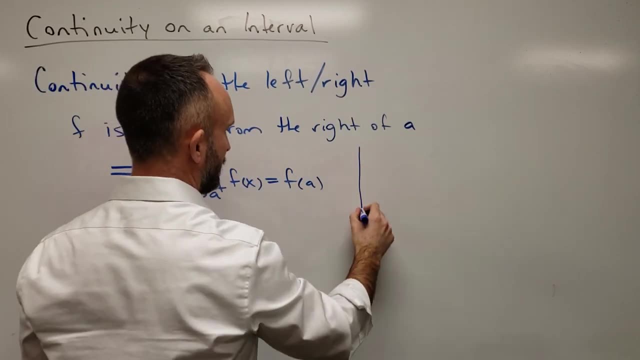 we approach a from the right, And if that limit equals the output of the function, then the function is continuous from the right of a. So a picture of that might look something like this: Say: say, this is your a value right And your function does this. 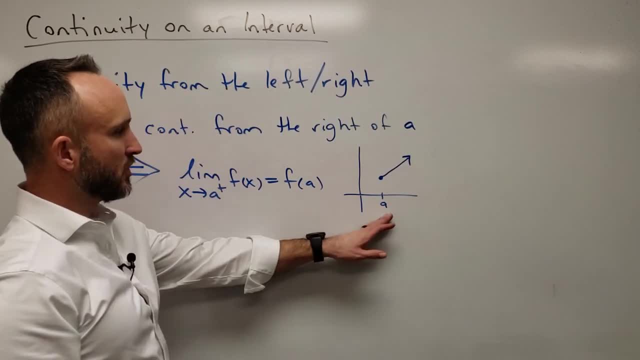 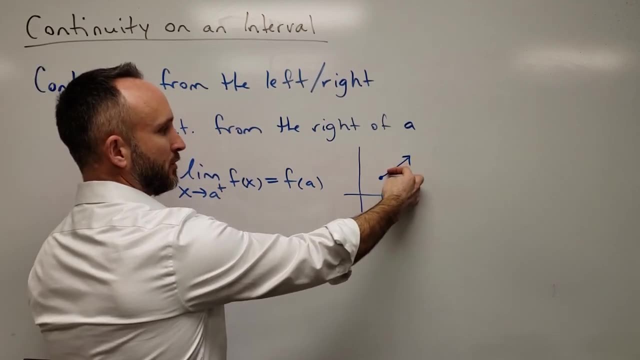 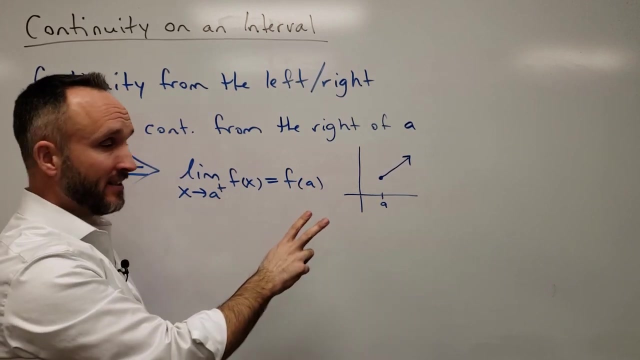 kind of thing. This function is continuous from the right of a Because as x approaches a from the right, we keep getting closer and closer to the actual output of the function at a. Now it's not continuous at a from both sides, because if f approaches a from the right, we 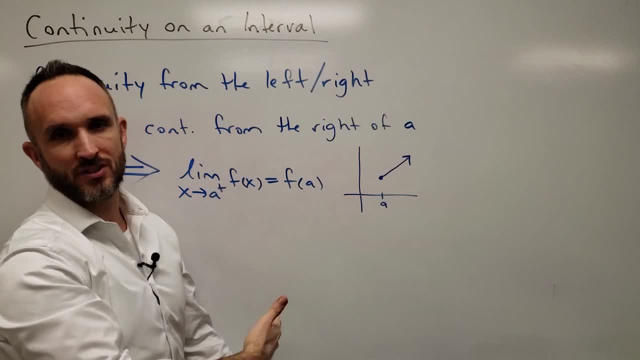 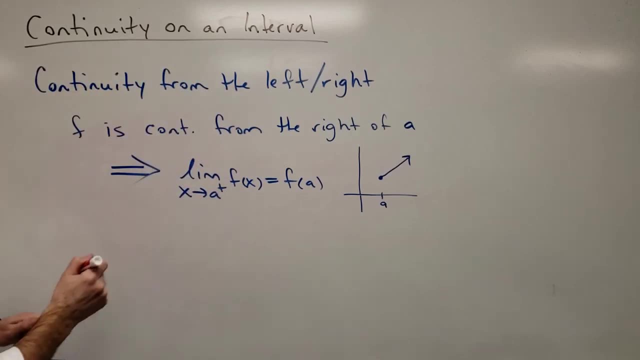 Because the left side of the limit doesn't even exist. The function is not defined on the left side of A, So similarly we could do the same thing from the left. So I'll put: I don't need to rewrite all of this. 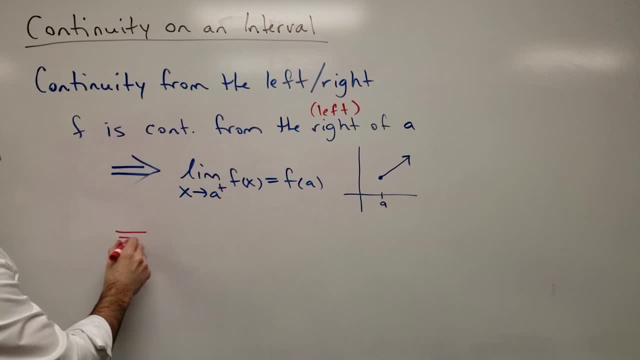 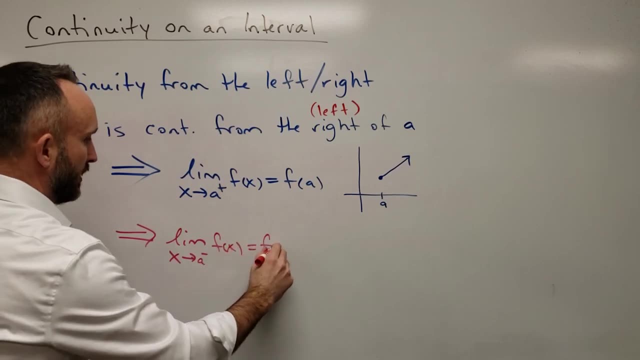 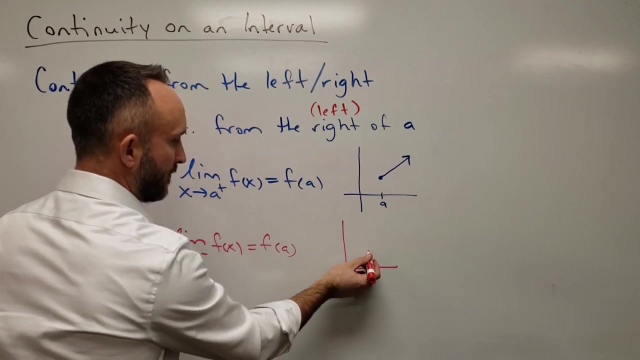 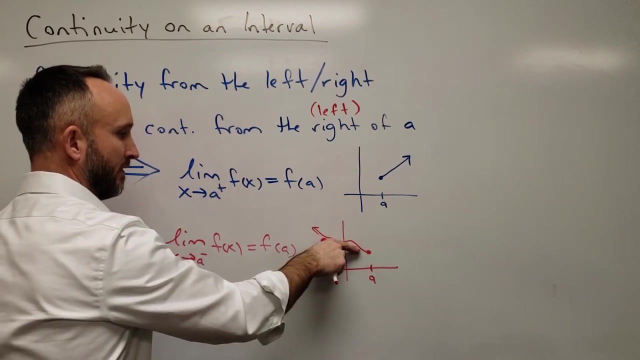 So F is continuous from the left of A. if the limit as X approaches A from the left equals the output at A And you can imagine a similar type of graph. if this is A, then maybe the graph does something like this: right, As X approaches A from the left, we keep getting infinitely close to the actual output at A. 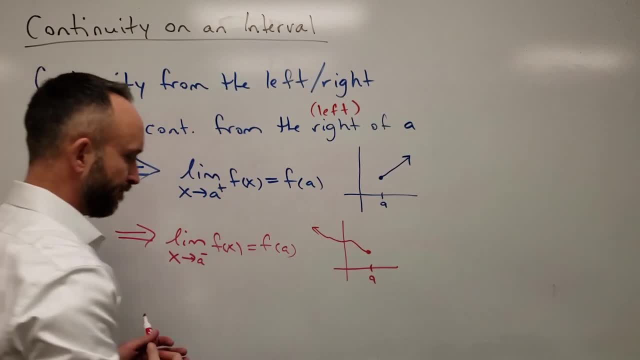 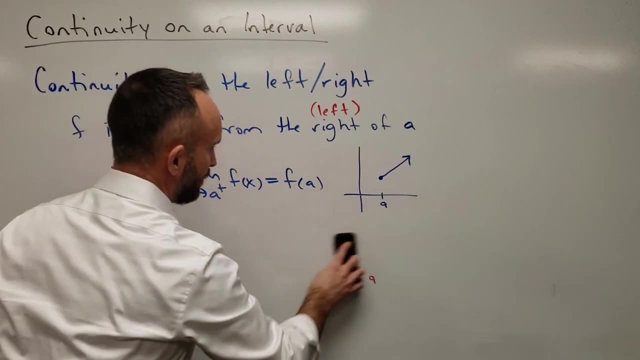 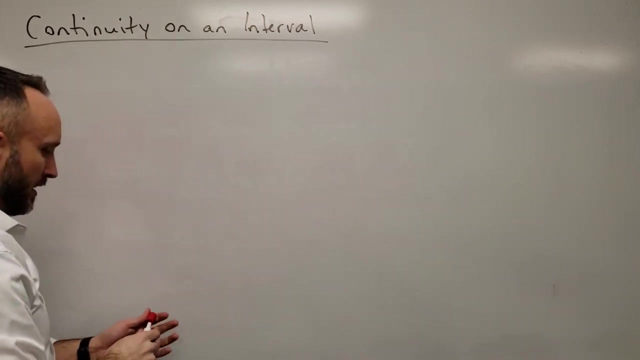 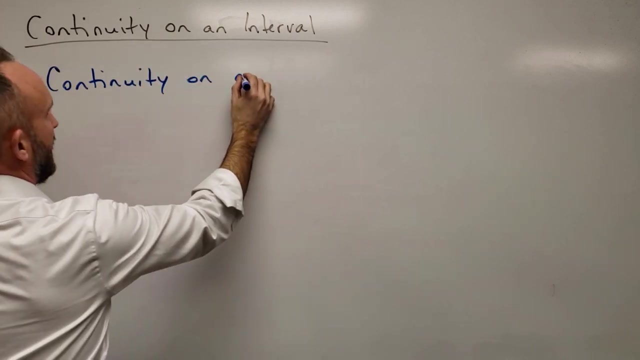 All right. so that's left and right continuity. No big deal, But that is key to understanding continuity on intervals. okay, So let's start with the simplest type of interval. Let's start with an open interval: Continuity on an open interval. 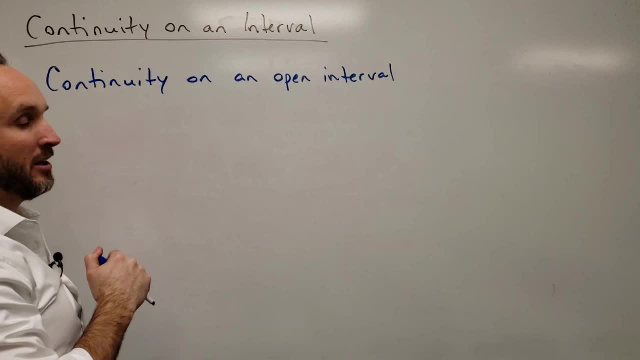 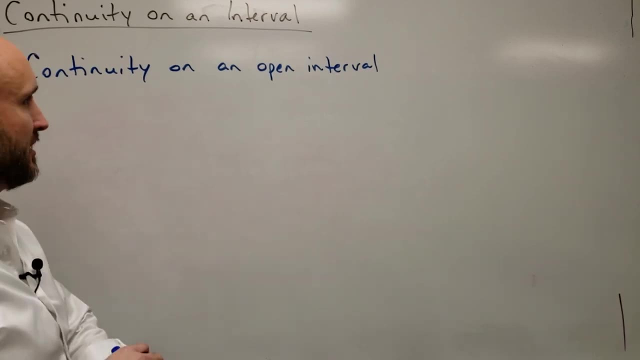 And these terms- open and closed intervals- need to become very familiar with. They'll be used in a lot of theorems and a lot of definitions throughout calculus And various forms of analysis, if you go on further with your education. So continuity on an open interval. 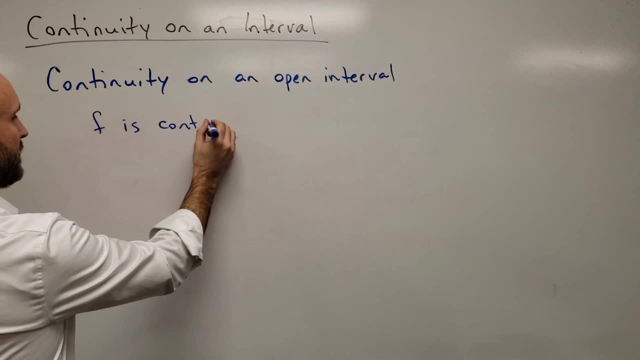 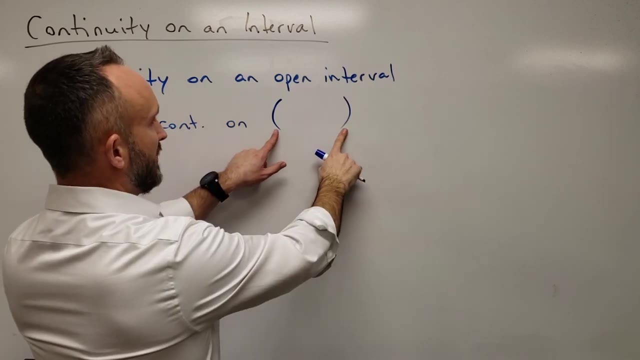 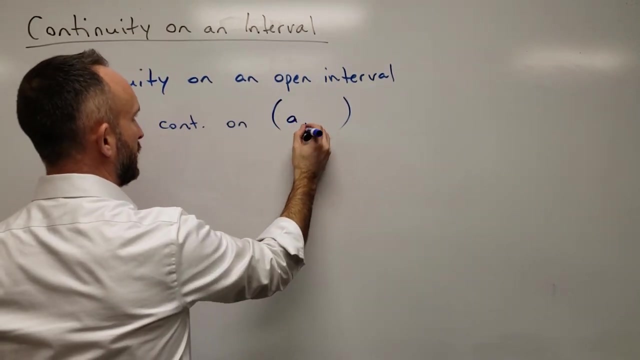 So we say F is continuous on an open interval means it's an interval of numbers where the endpoints of the interval are not included. So you use parentheses. It's interval notation is what it is. So F is continuous on the open interval from A to B if 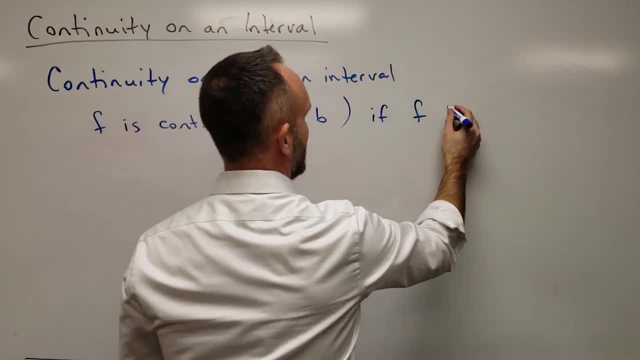 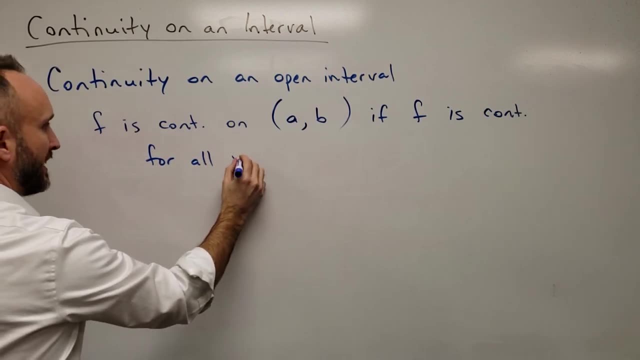 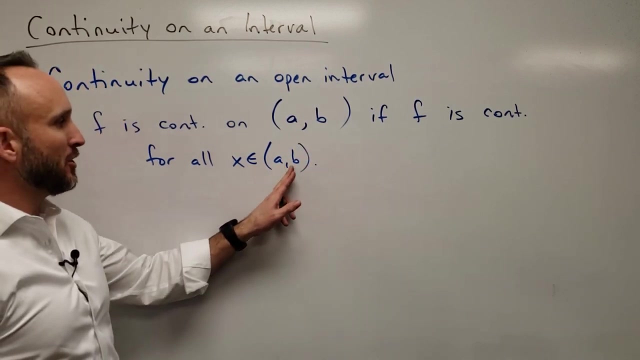 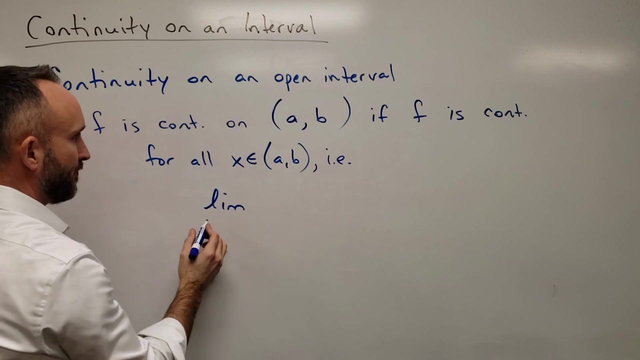 F is continuous. if F is continuous for all, for all X values in that open interval, okay. So if you pick any value in here, so in other words the limit, let's call this X sub zero, X naught, Okay. 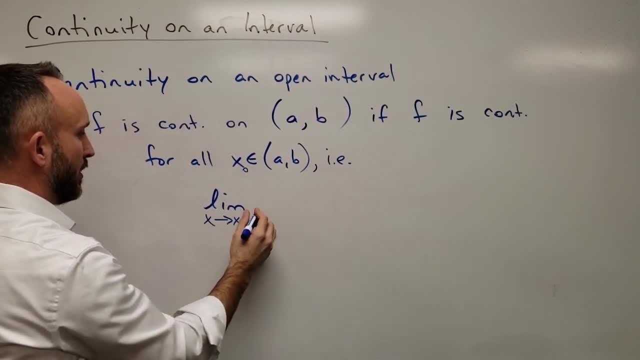 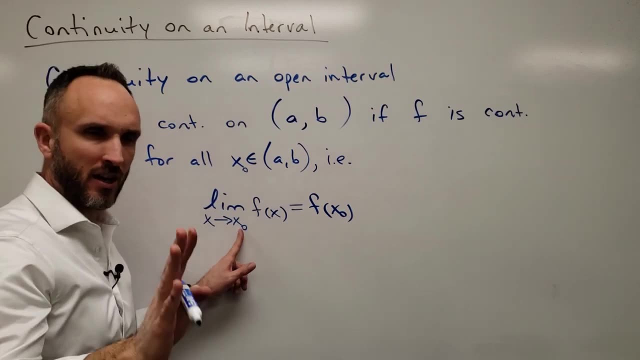 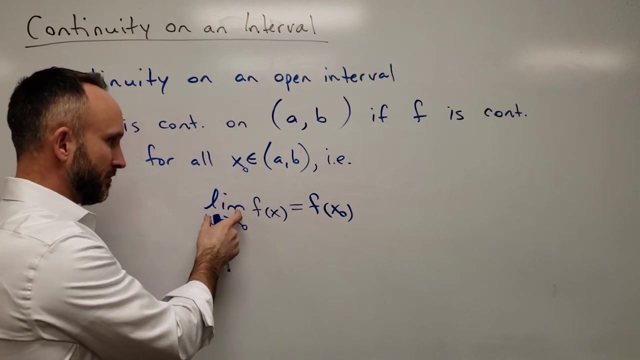 As X approaches X sub zero of F of X, that should equal F of X sub zero. right, X sub zero is a constant. okay, Any constant in this interval is: X gets close to that. The limit of the Y values gets close to the output at that constant. 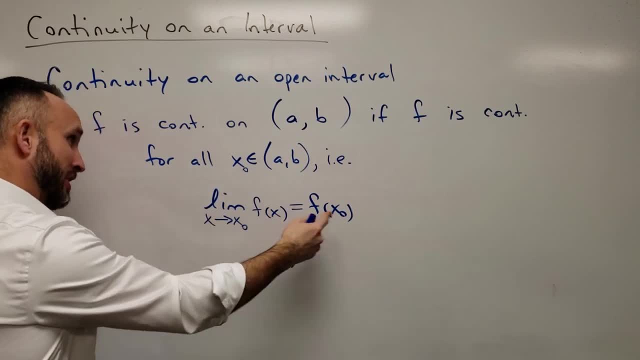 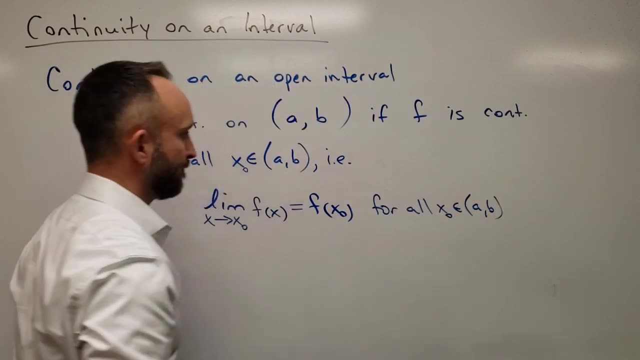 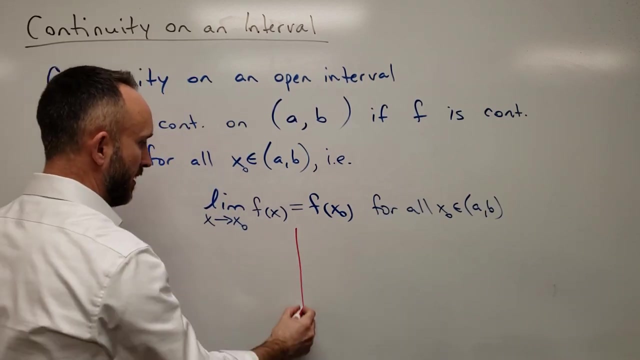 This is the definition of continuity at a value. This should be true For all X naught in the interval from A to B. Okay, So no big deal. If you were to draw a picture of a graph of this, maybe it would look like let's say, here's A, here's B. 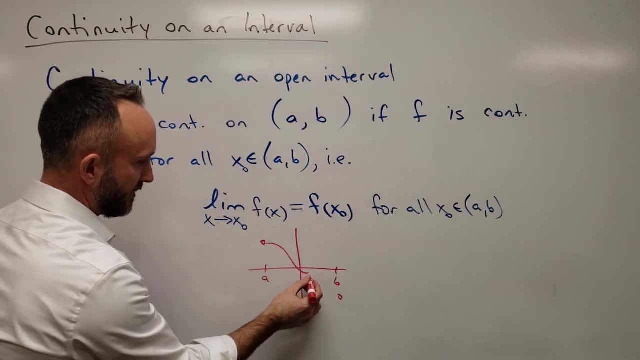 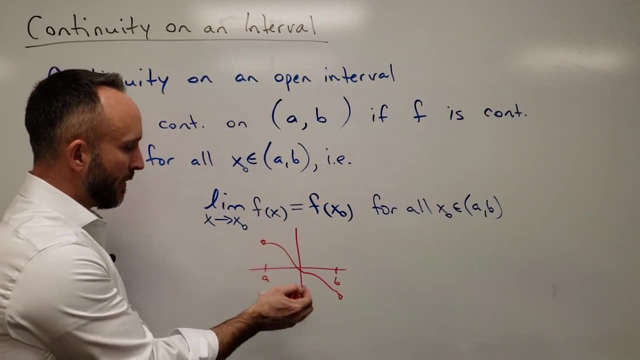 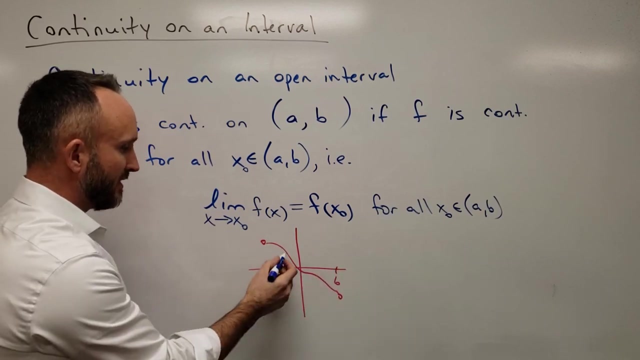 and open circle there, open circle there, and your graph does this type of thing. So this function is continuous on the open interval from A to B, because no matter what X sub 0 that you choose, no matter what x sub 0 you choose between these, the limit from both sides. 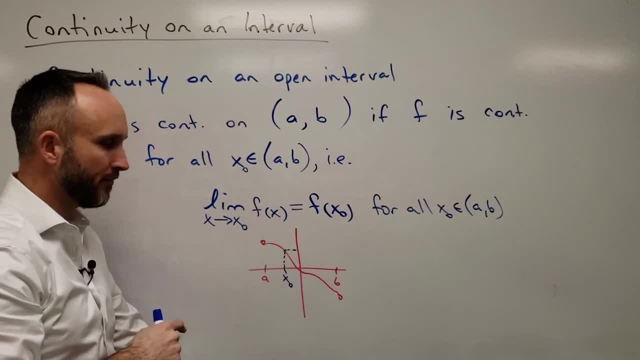 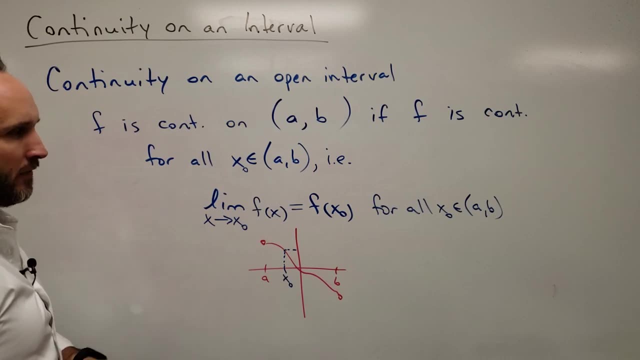 equals the output of the function. There's no gap right there. In fact, that's true for any x sub 0 between a and b. Okay, so that's continuity on an open interval. Very simple, It just means it's continuous at every point in that interval, every x value in that interval. Let's look at: 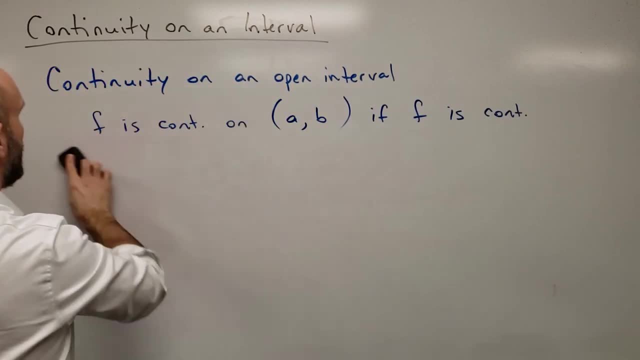 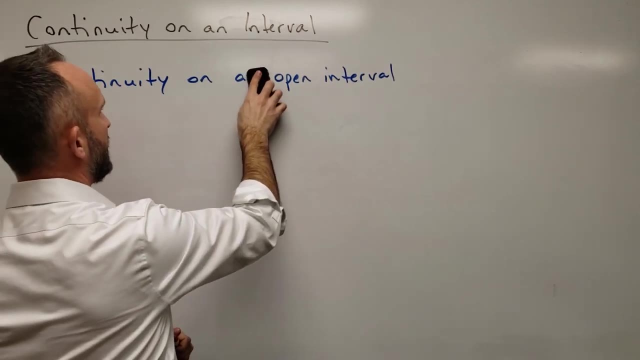 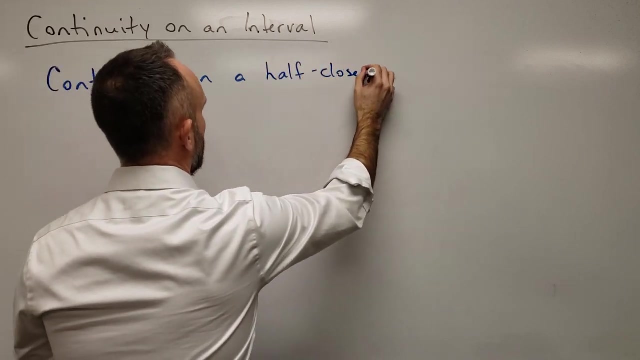 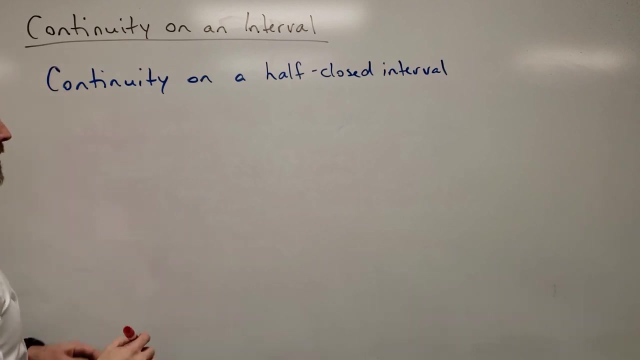 continuity on, let's call it a half-closed interval, continuity on a half-closed interval. And so the way we'll describe that is we'll say f is continuous. f is continuous. continuous on this interval. Let's say it starts out open, it's half open, but then it's closed. 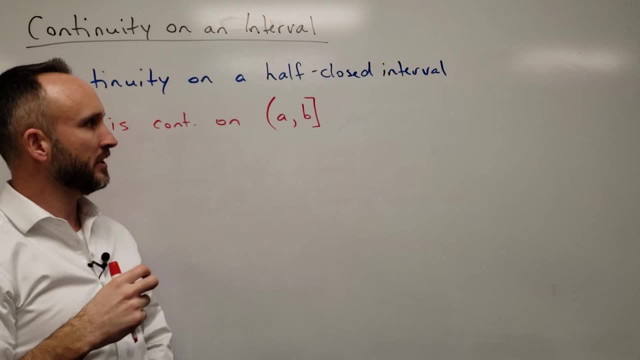 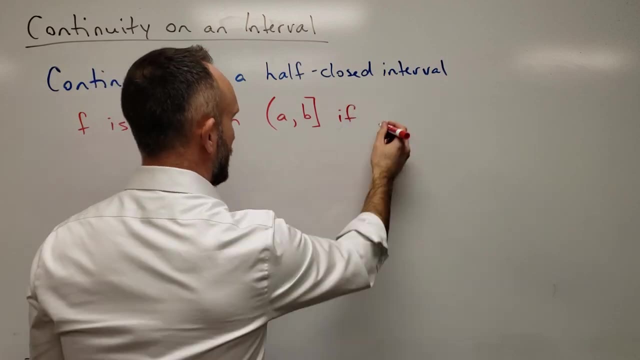 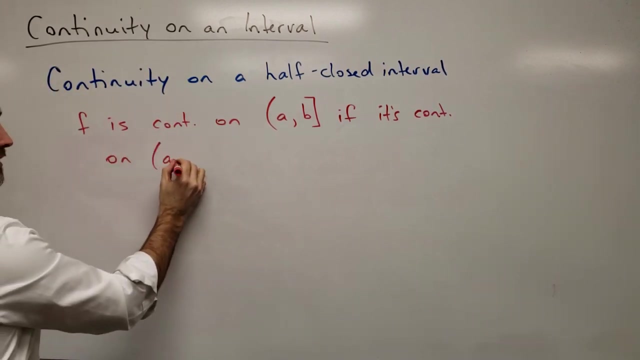 at b. All right, so that's not a completely open interval. We'll call it half-closed. So f is continuous on this interval. if it's continuous on the open interval, right? In other words, it's continuous for every value between a and b. 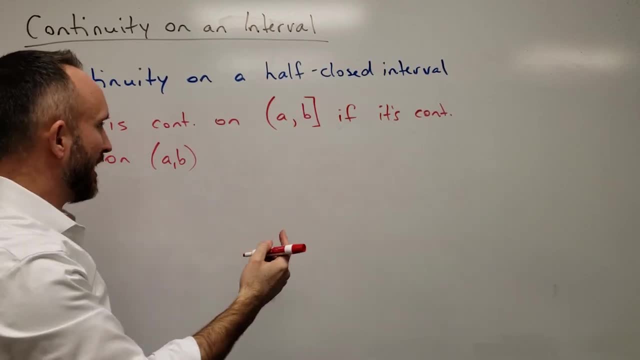 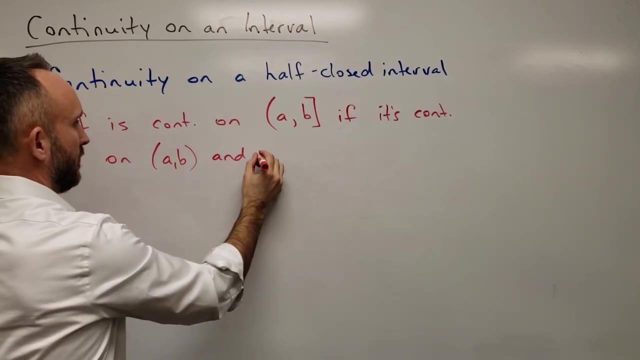 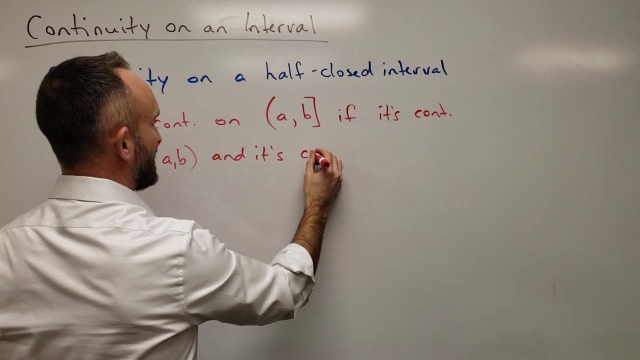 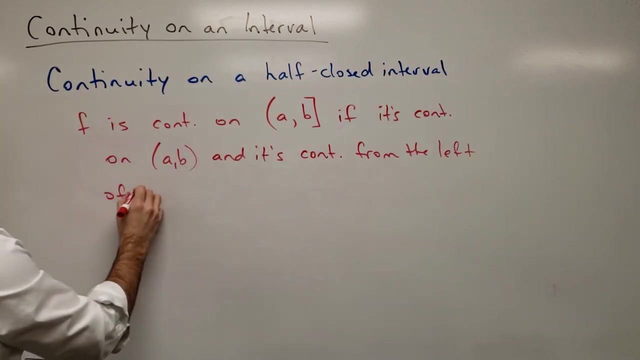 And then what about b? though B should be included somehow, So when you have an end point of your interval that's included, then in this case, since the function is defined to the left of b, it has to be continuous from the left of b. All right, So it's continuous for everything. 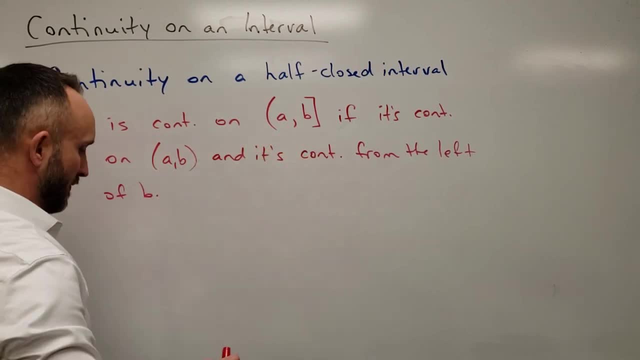 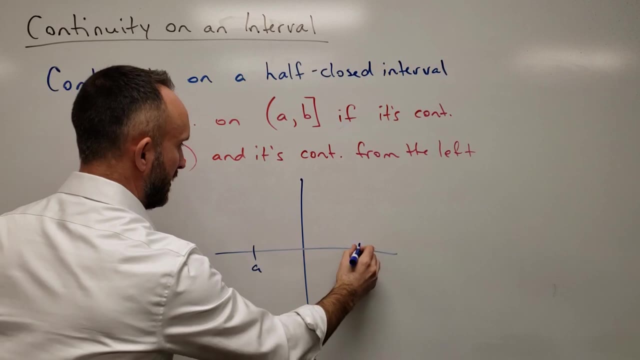 between a and b and then it's continuous for the left of b. So that's a half-closed interval is from the left of B. So if you were to draw a picture of this, let's say here's A, here's B, we might have an open circle. then it's all smooth, no gaps. 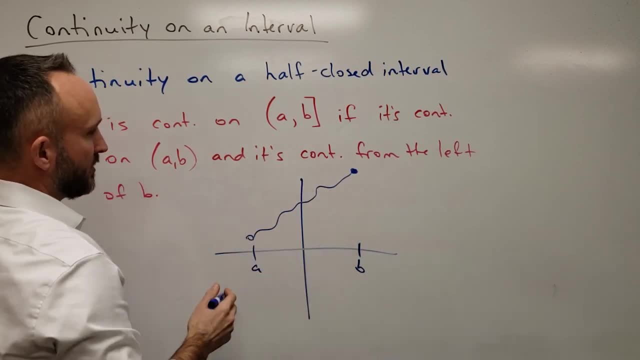 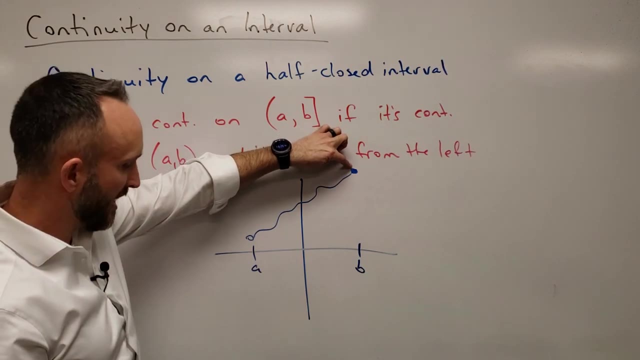 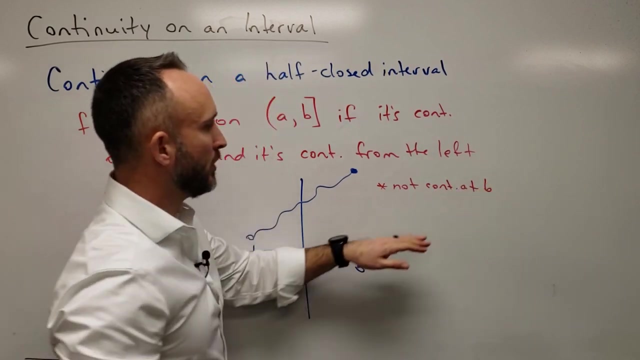 and then when it gets to B, it's a closed circle. So you could pick any value between A and B and you can see it's continuous. Now notice: this function is not continuous at B, Not continuous at B. When you say a function's continuous at a value, that means from both sides. 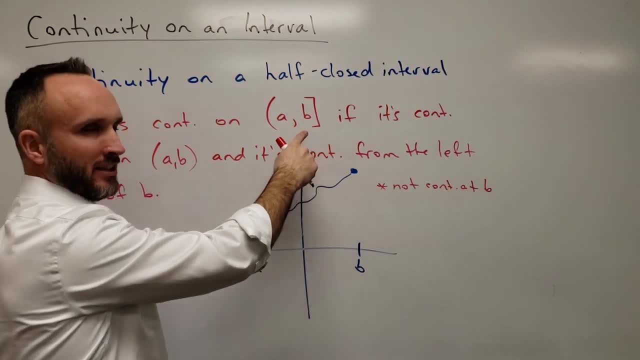 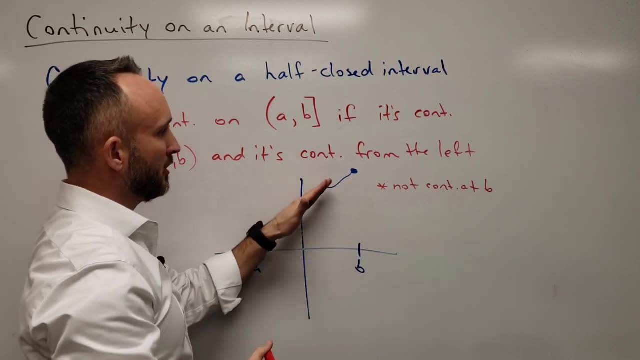 So if your endpoint has a bracket it's not necessarily continuous from both sides, but we know because it's the right endpoint, it better be continuous from the left So your limit approaches your output from the left only. okay, So it's continuous between. 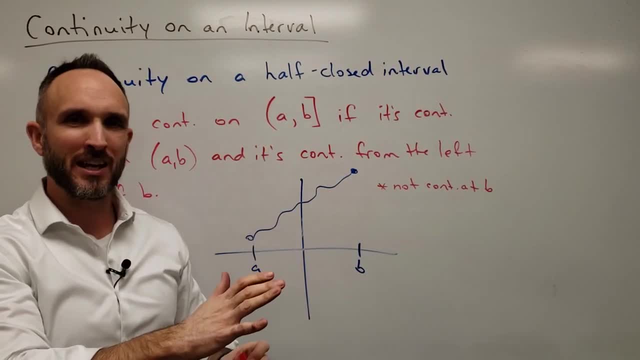 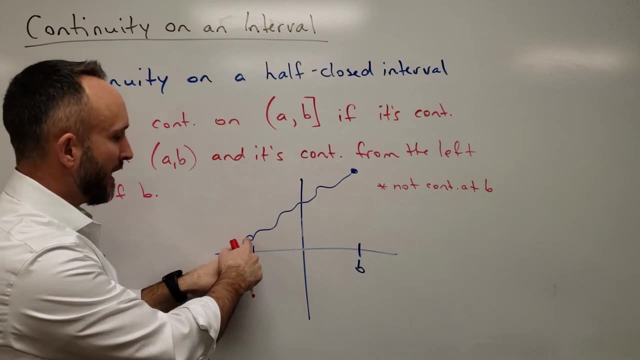 and from the left of your right endpoint. You could do the same thing with a half closed interval where your left endpoint is included. This would be a closed circle. You'd have to say it's continuous from the right of that endpoint. So I won't write all that down. 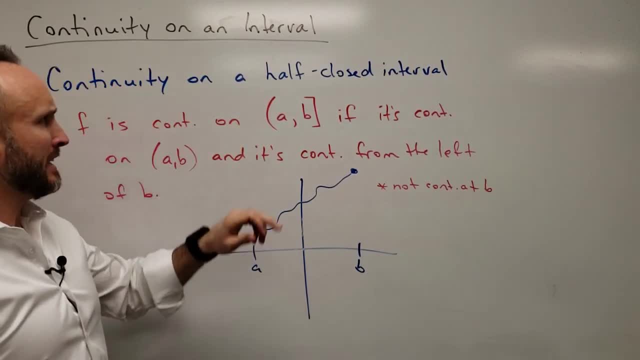 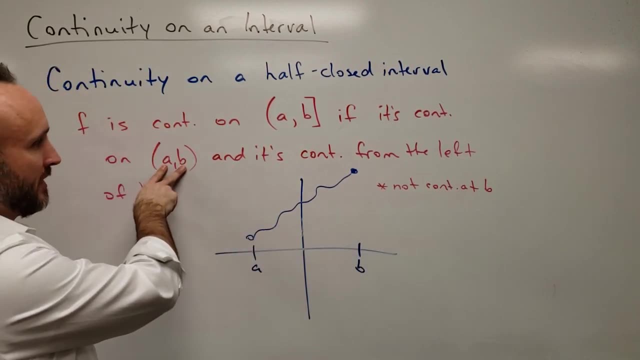 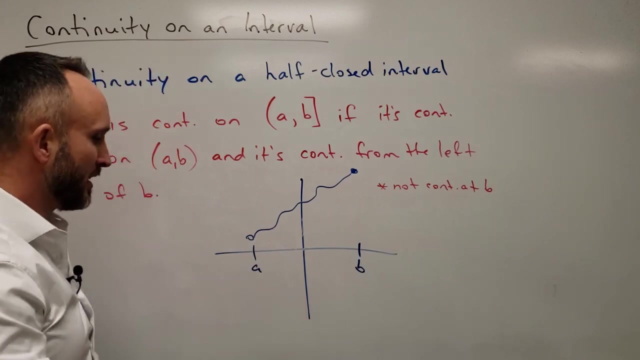 It's the same idea. I also won't write down a fully closed interval, because that's similar. It'll be continuous between. so it'll be continuous on the open interval and it's continuous from the right of the left endpoint and from the left of the right endpoint. okay, So that's continuity on. 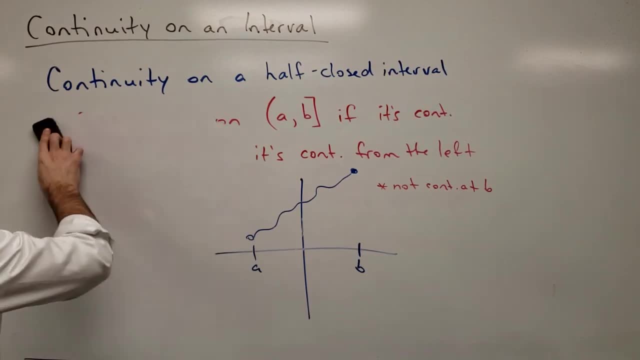 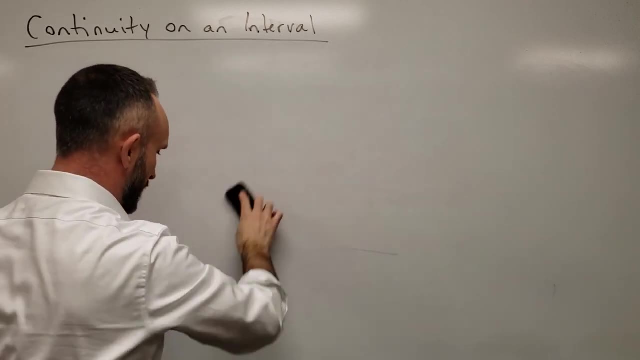 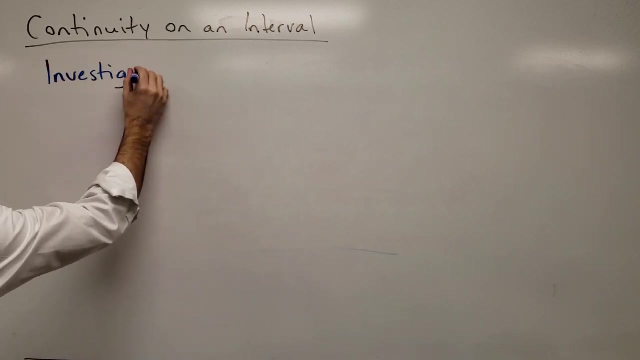 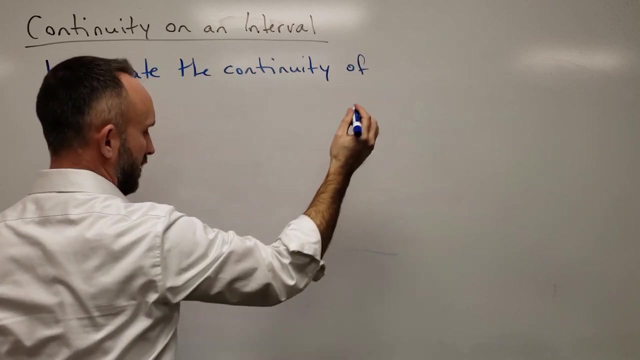 various types of interval. So if you're going to draw a picture of this, you're going to have to- of intervals. Let's look at a really good example of this. Investigate: the continuity of f of x equals the square root of f of x. So if you're going to draw a picture of this, you're going to have to. 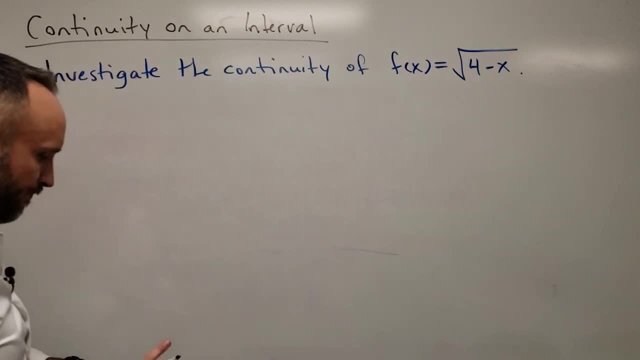 of 4 minus x. okay, So in this case we know that if I want the limit of this function, so if I pick any a value in the interval, this, by the way, means is an element of or is in, If I pick any a in the interval. 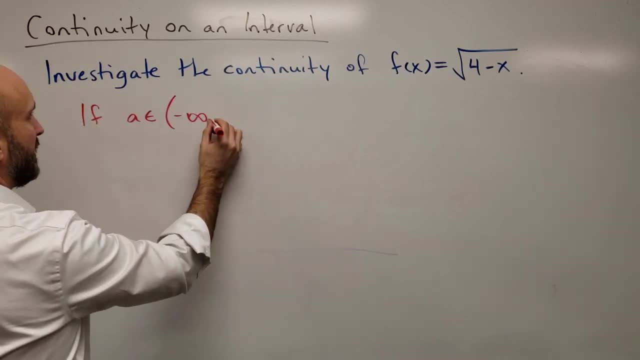 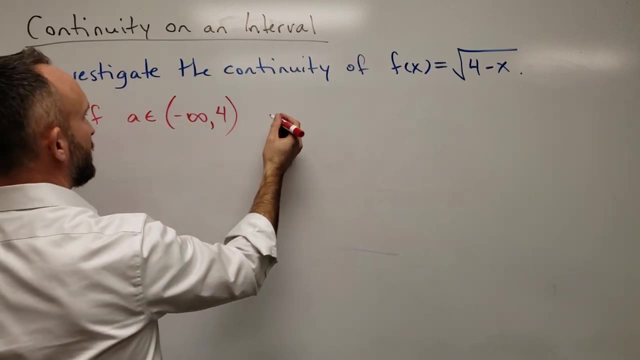 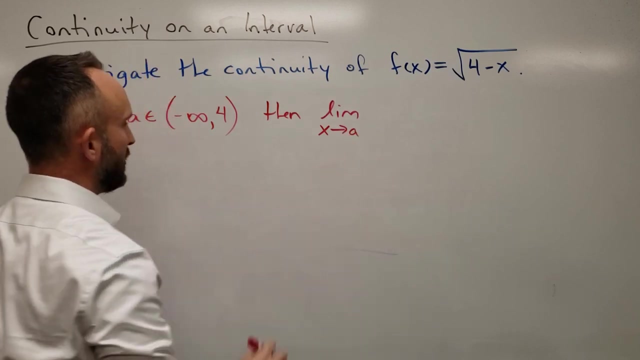 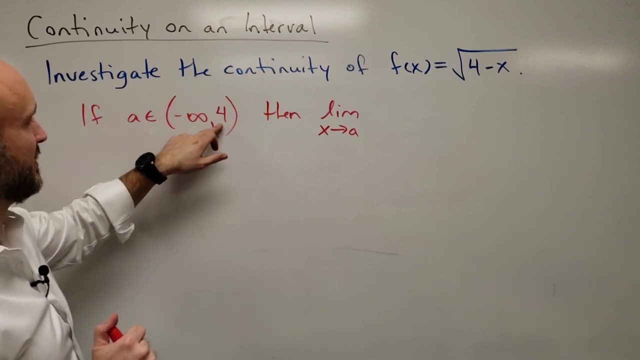 the interval from negative infinity to 4.. Let's not include 4.. No matter what a value I choose here, then the limit as x approaches that a value. you can investigate some of these. For example, I could choose 2, right for my a value because 2 is in this interval If I take the limit as x approaches any of those a values. 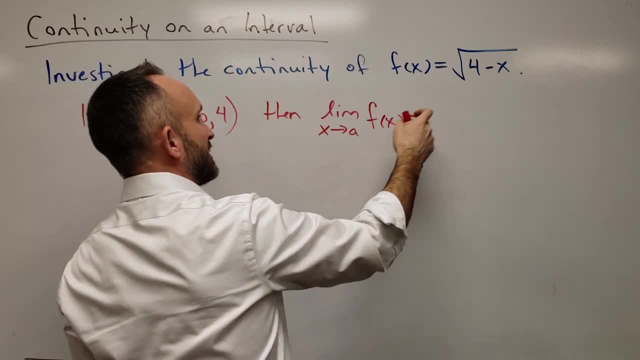 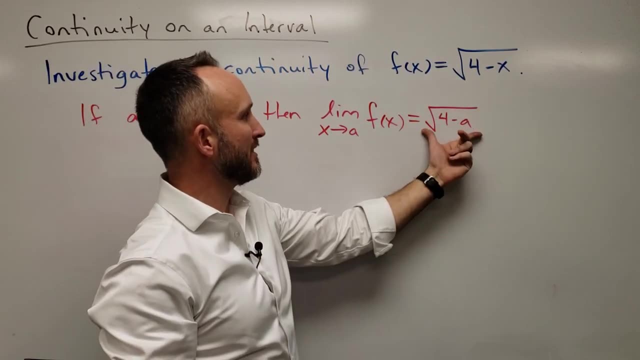 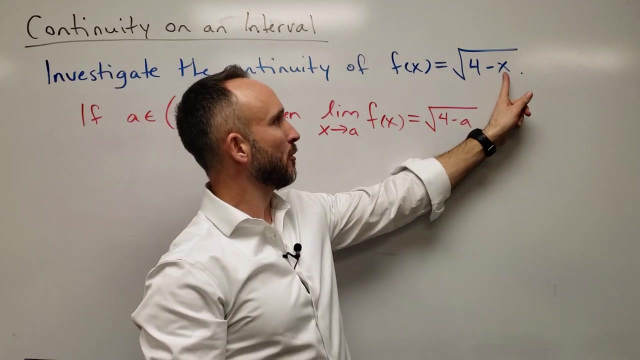 then I can. I can take the limit by doing direct substitution. I can plug my a into the function to get the limit, because this will calculate nicely. I don't have any issues. the only issues I'd have is if I were plugging in a number bigger. 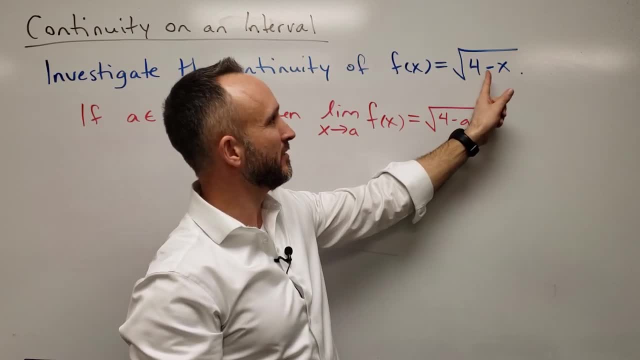 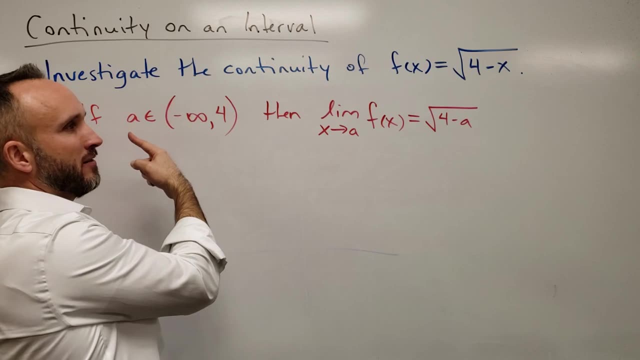 than 4, because 4 minus something bigger would be a negative and a square root of a negative would be imaginary. that limit would not exist. but as long as I choose numbers smaller than 4, I don't have to worry about that. so, in other words, as X. 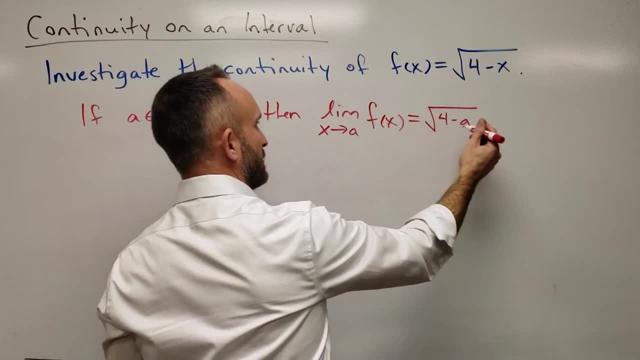 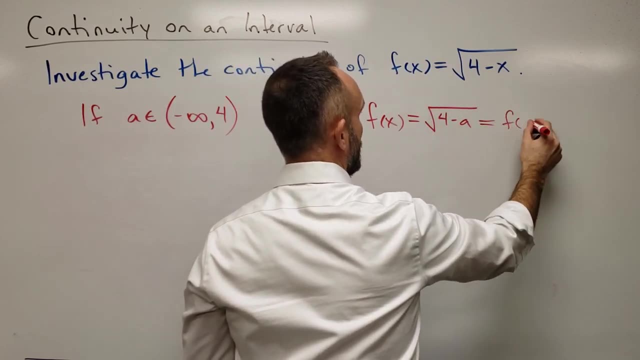 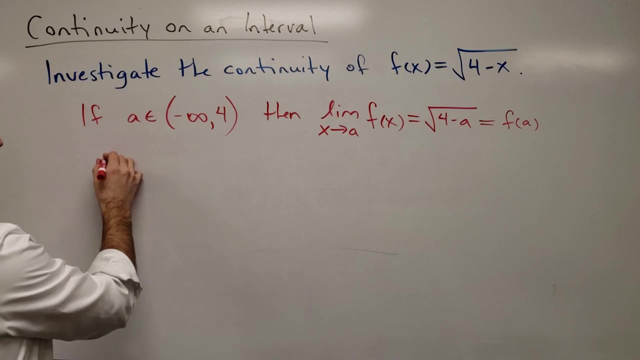 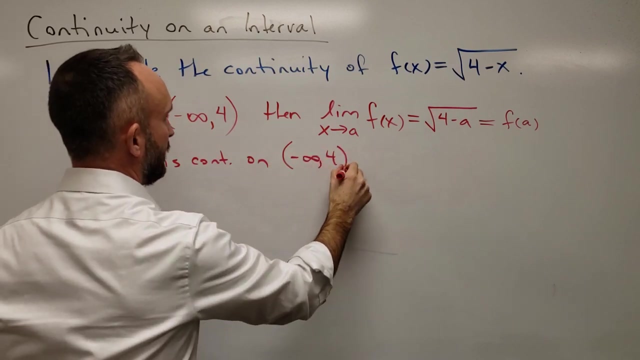 approaches any of these a values. I can calculate it by direct substitution, and the square root of 4 minus a is literally the same thing as F of a. by definition it's it's the function evaluated at a, so therefore F is continuous on this open interval. 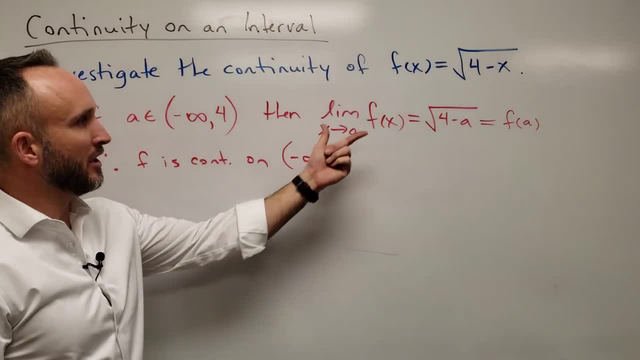 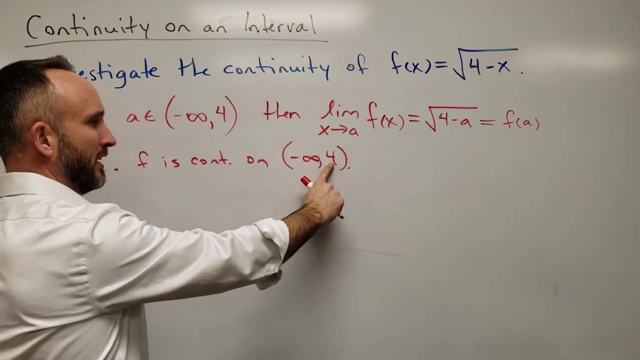 right, I could pick any value from this interval and I know it's continuous at those values, so it's continuous on the interval. but you can see the end point of 4. let's investigate what happens at 4. we already know that we can't choose. 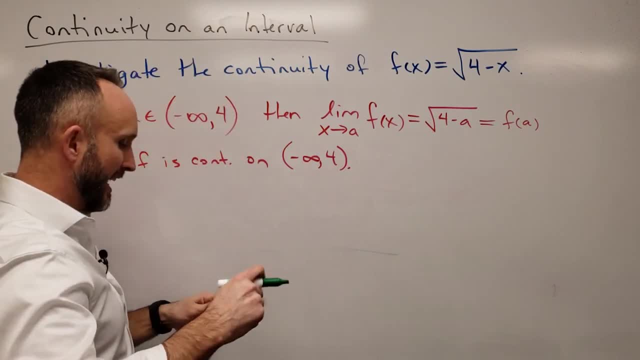 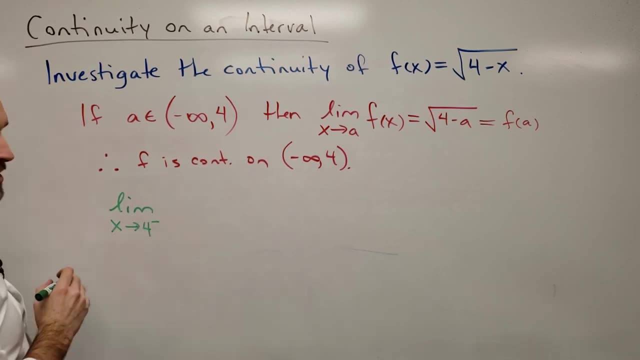 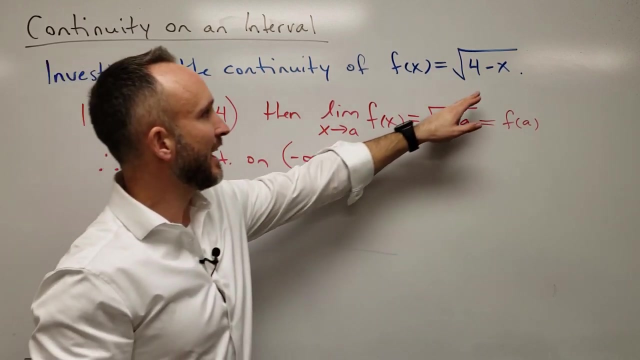 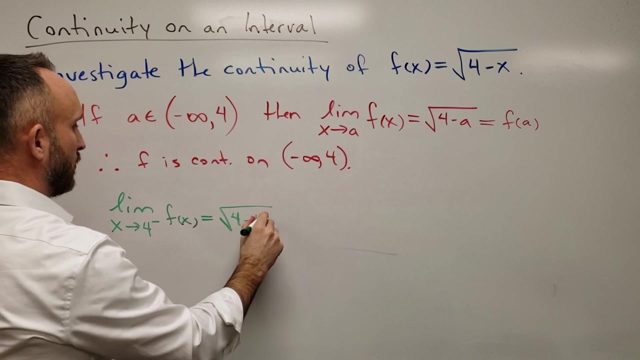 numbers to the right of 4. so let's look at the limit, the limit as X approaches 4 from the left. let's choose numbers slightly less than 4. well, as long as I choose numbers less than 4, I can calculate my limit by direct substitution. so that's going to be the square root of 4 minus 4, which is: